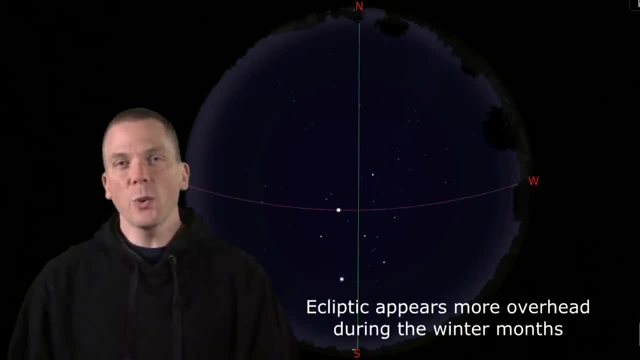 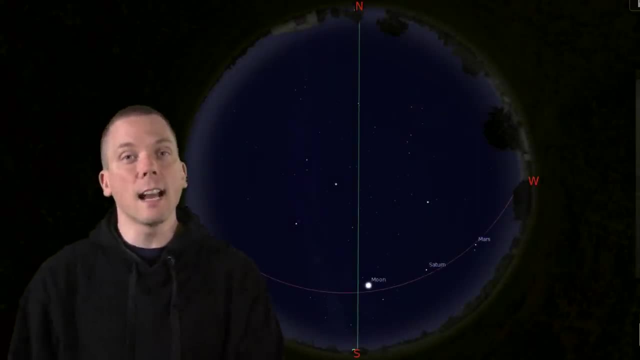 the ecliptic starts with the sun and adds up to the planets near the sun's centre, Then the winter months at night. So close to, or sometimes right on the ecliptic is where we will always find the naked eye and telescopic planets in our solar system and the moon. 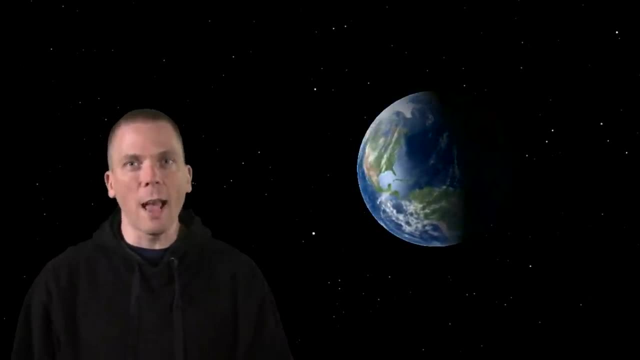 Keep in mind that the sun doesn't actually rise or set. what's actually happening is the Earth is rotating. We just don't feel that rotation because we humans are just along for the ride. So as Earth spins, imagine if you were standing at the North Pole. 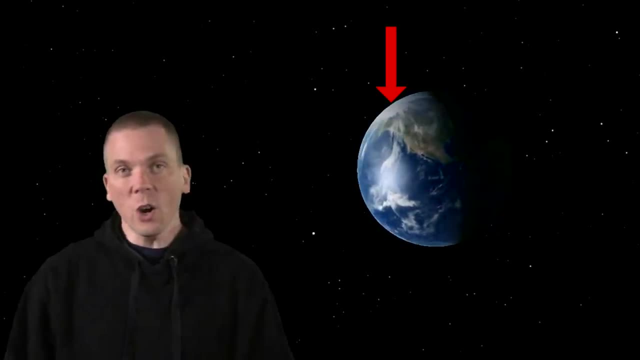 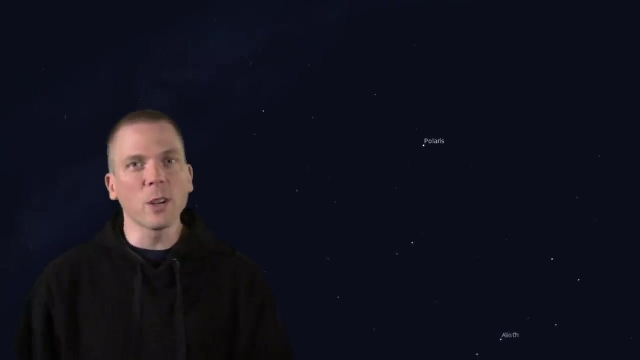 and looked straight overhead. when it was dark, The stars would appear to spin around a circle, and the axis of that circle- at the zenith, the point overhead we talked about earlier, That point in the sky around which the stars rotate, is the Celestial Pole, Of course. 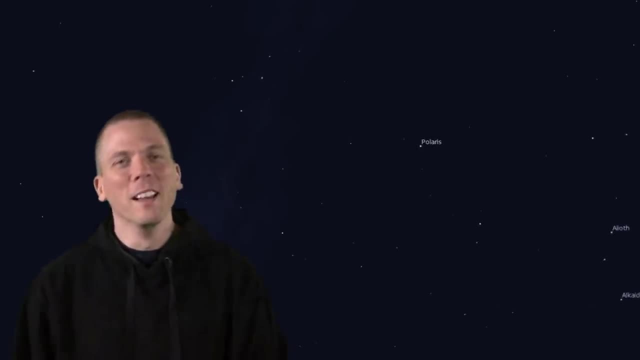 you likely won't ever see that because no one lives at the North Pole. So as we move downwards in latitude in the Northern Hemisphere, that point in the sky around which the stars rotate will move downwards, Down towards the north part of the horizon. If you're in the upper latitudes, it will appear. 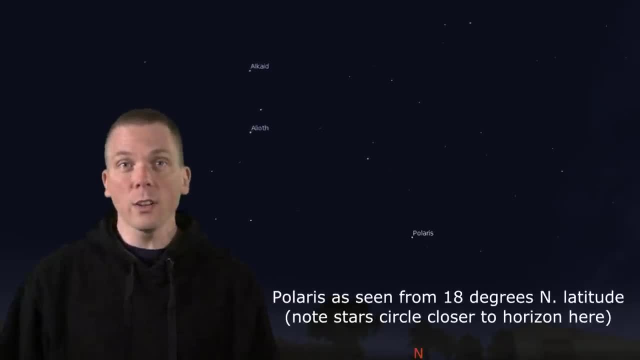 higher in the sky. The nearer you are to the equator, the closer that point is going to be to the northern horizon. If you've ever looked at a globe with latitude and longitude lines on it, you can probably imagine pretty easily our next set of markings in the sky. 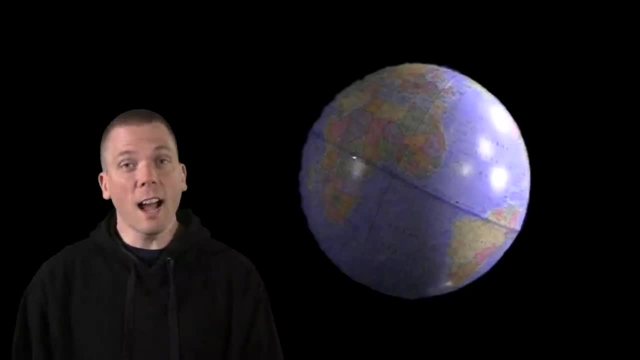 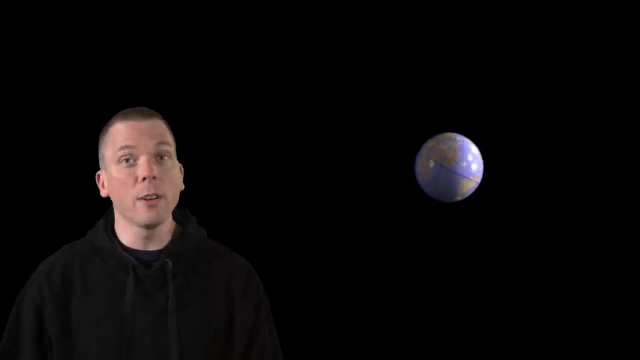 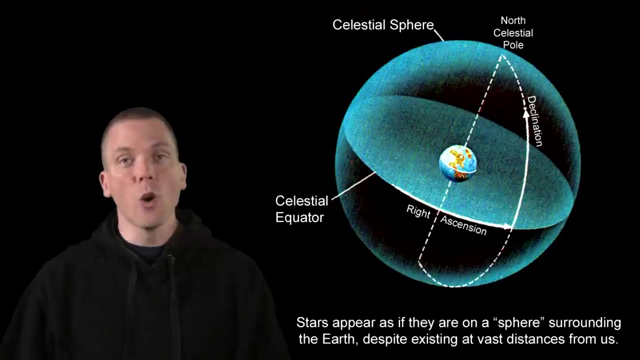 the Celestial Sphere. To locate objects in the sky, we use coordinates like on Earth, instead of latitude and longitude, and project those lines out past space as if they were on a transparent sphere surrounding Earth. These are right ascension and declination. Right ascension is actually easy to remember. 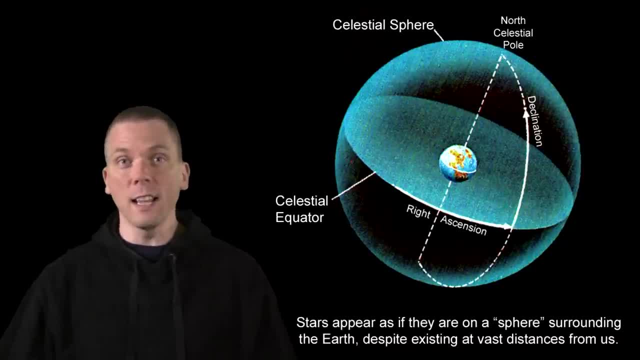 if you face north and the Sun rises east, which side of your body is that on? Well, it's on the right side, So the Sun ascends from your right or right ascension. These are longitude lines on Earth that start at one pole and run to the other pole in equal spacings.